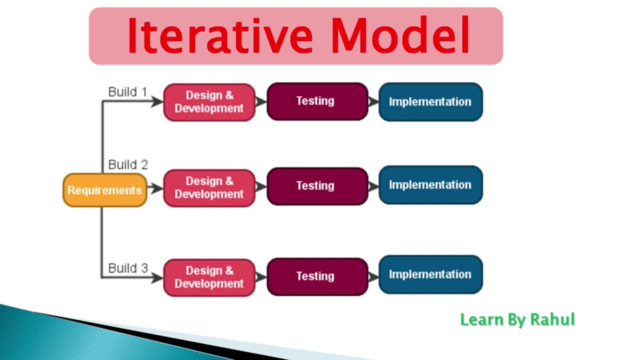 So that's why iterative model comes in the picture. Let me take example to understand iterative model in a very simple way. If you want to make a painting, so first you sketch it, then again implement or do new changes or design, Then add some color to look more attractive. or we can say in the first step: 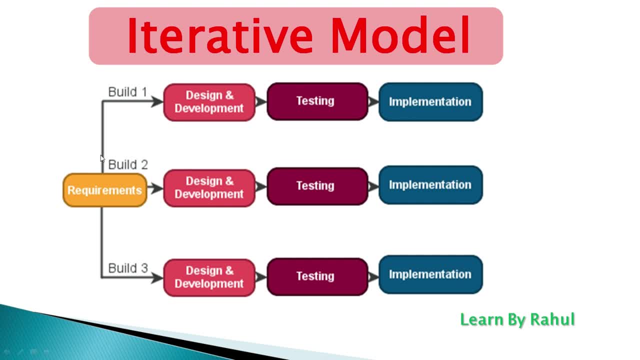 In the first iteration the whole painting is sketched roughly, Then in the second iteration colors are filled, and in the third iteration finishing is done. Hence, in iterative model the whole product is developed step by step. Or we can say: when we work iteratively, we create rough product or product piece in one iteration. 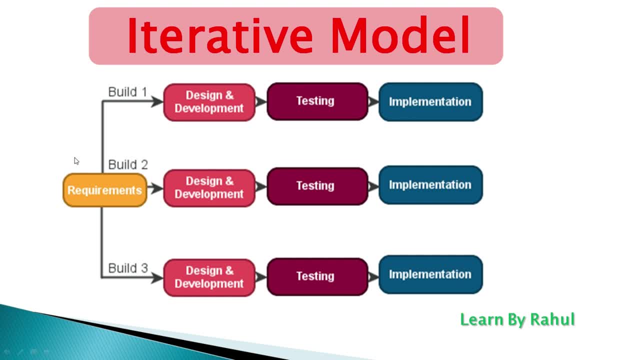 Then review it and improve it in the next iteration, So and so on until finished. Or we can say the iterative process model in the implementation of the software development life cycle, in which the initial development is started based on the initial requirement And more features are added to the base software product, with the ongoing iteration until the final system is created. 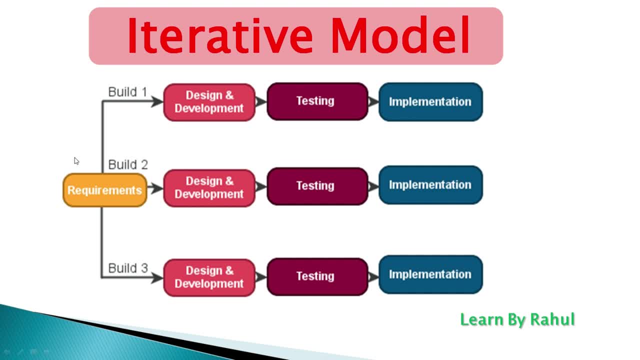 An iterative life cycle model does not attempt to start with a full specification of requirement. Instead, development begins by specifying and implementing just part of the software, Which can then be reviewed in order to identify further requirement. This process is then repeated, producing a new version of the software for each cycle of the model. 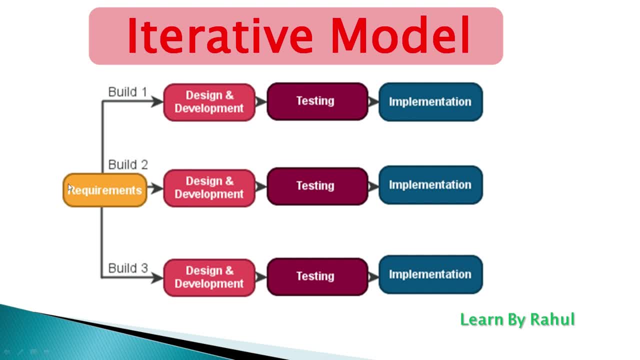 Now let's understand step by step iterative model. First we gather requirement from the customer. Then we design the software and develop it. Then tester test the application. If he find any issue he again contact back to the developer. Then developer fix that issue and tester again test the entire application. 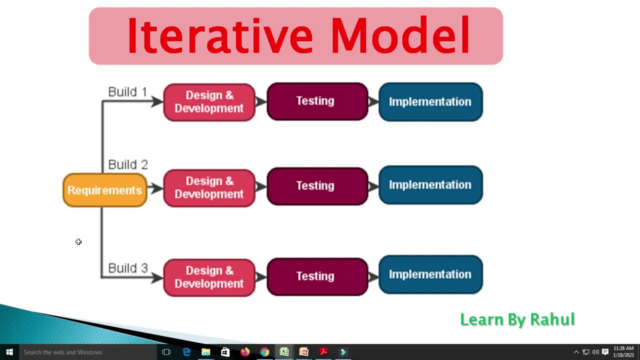 The last phase is implementation. It is the most important phase of the iterative model. Here the actual implementation and coding process is executed. All planning, specification and design document up to the points are coded and implemented into this initial iterative of the project. The requirement then design. 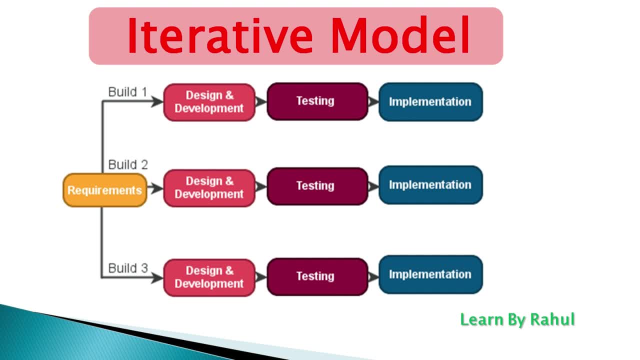 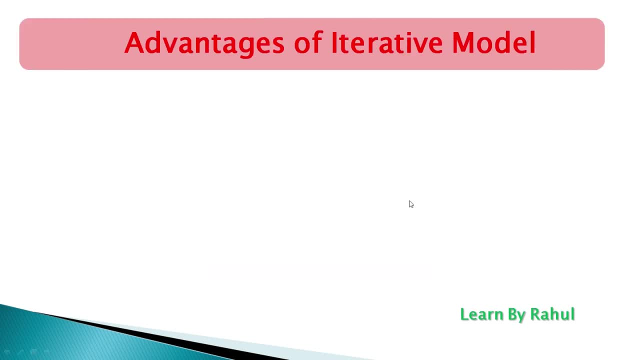 Development, Testing and again implementation. So we do all process again and again. That is why it is called iterative model. Let's we talk about advantages of iterative model. The end user or the stack holder can give their feedback quickly, Which can then be implemented into the system. 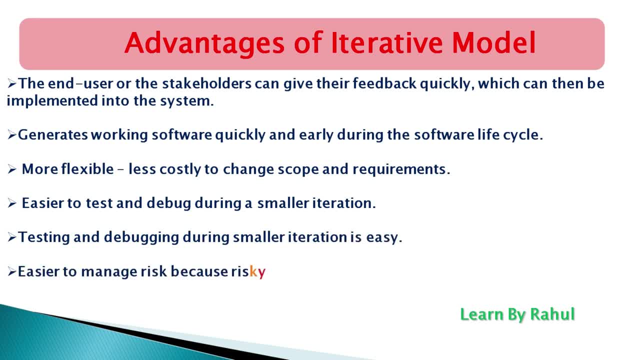 Generates working software quickly and early during the software life cycle. More flexible, Less costly to change scope and requirement. Easier to test and debug during a small iteration. Testing and debugging during small iteration is easy. Easier to manage risk because risky pieces are identified and handled during its iteration. 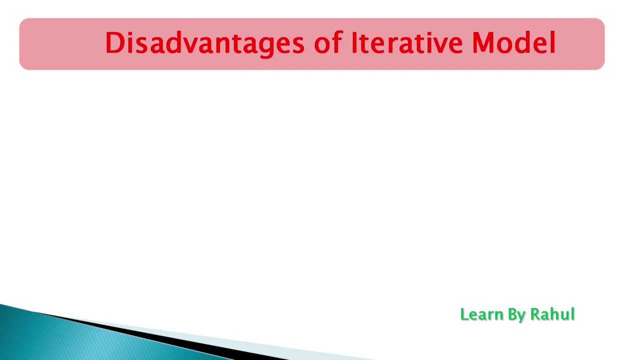 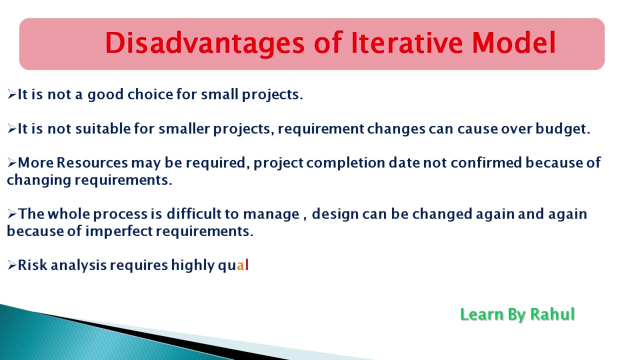 Each iteration is an easily managed milestone. Let's we talk about disadvantages of iterative model. It is not a good choice for small projects. Second, it is not suitable for small projects required. Small projects requirement changes can cause over budget. Third, more resources may be required. 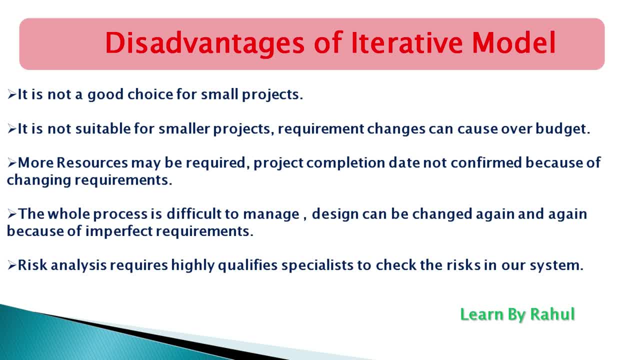 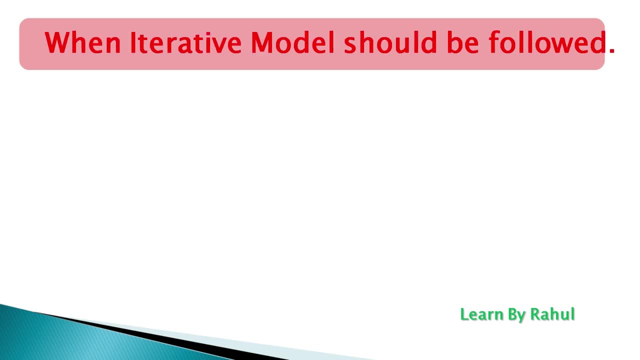 Project completion date not confirmed. because of the changing requirements, The whole process is difficult to manage. Design can be changed again and again because of imperfect requirement. Last, risk analysis requires highly qualified specialist to check the risk in our system. Let's we talk about when iterative model should be followed. 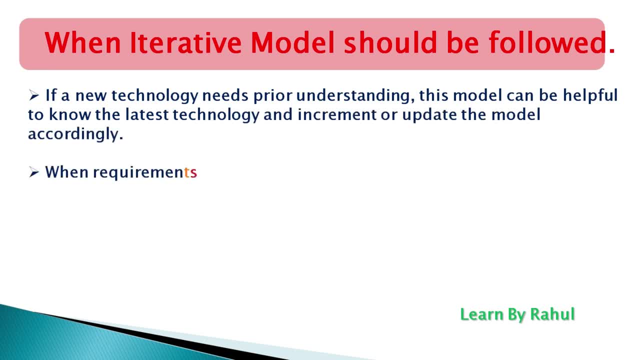 The first, if a new technology needs prior understanding. this model can be helpful to know the latest technology and increment or update the model accordingly When requirements are defined clearly and easy to understand. Third, if frequent changes required in the project. And the last when there is a requirement of changes in future. 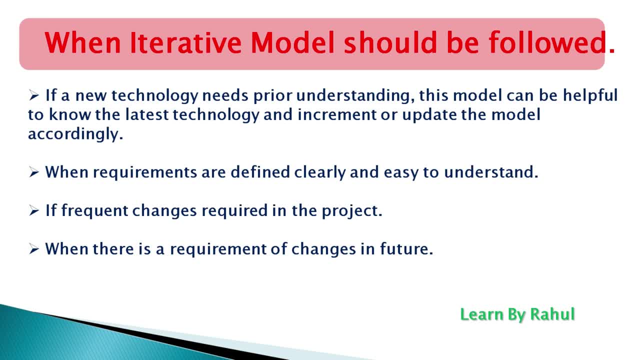 So this is all about iterative model and if you have any query, you can comment below, And for more videos and update, you can subscribe my channel, Thank you,